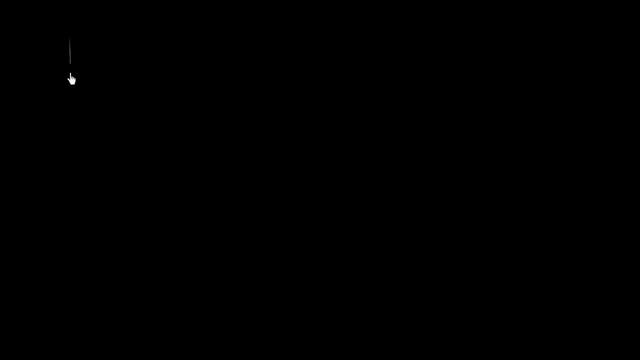 Let's say that we have a sheet of cardboard that is 20 inches by 30 inches. Let me draw the cardboard as neatly as I can So it might look something like that. So that is my sheet of cardboard And just to make sure we know the dimensions. 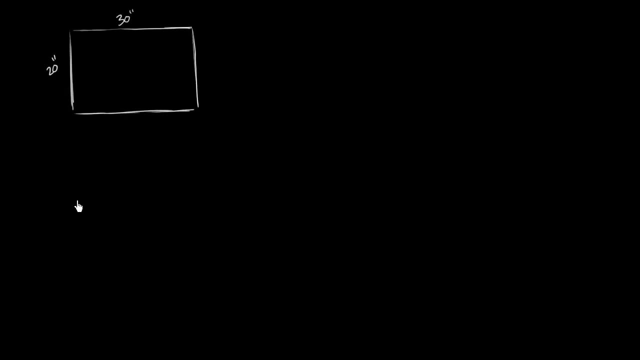 it is 20 inches by 30 inches And what we're going to do is cut out the corners of this cardboard, And all the corners are going to be squares, And we're going to cut out an x by x corner from each of the corners of this piece of cardboard. 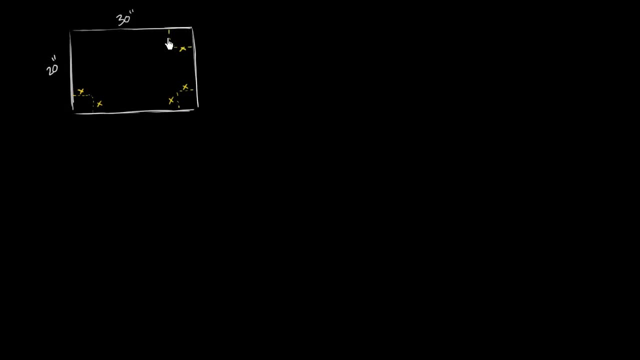 x by x, Over here, x by x, And then over here, x by x. And what we'll do is, after we cut out those corners, we can essentially fold down the flaps. Let me draw the flaps so you can imagine. 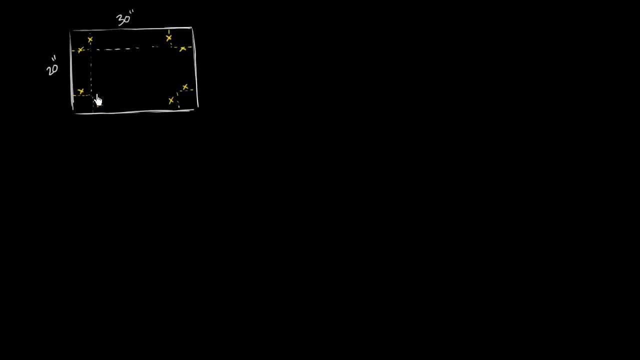 We can fold right there, We could fold right there, We could fold right there And we would form. I guess you could imagine a box without a bottom to it, Or you could view a box without a top to it. So if we were to fold everything up, 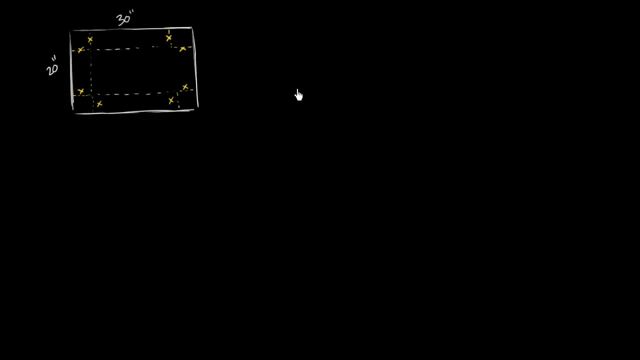 we would get a container that looks something like this. Let me make my best attempt to draw it So it would look like this. It would look like this: This is one flap folded up. You can imagine this flap right over here If I were to fold it up like that. 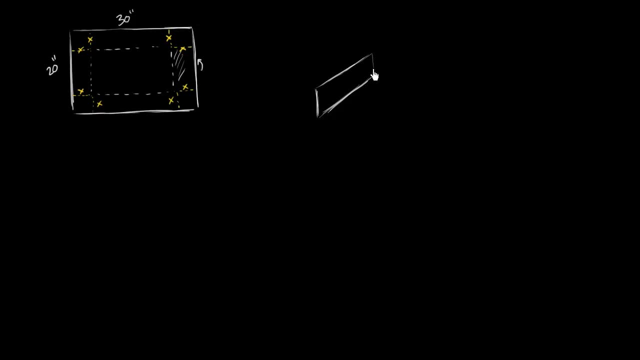 it now would look like this. It would now look like this: The height of the flap is x, So this distance right over here is x. And then if I were to fold this flap, if I were to, let me do that a little bit neater. 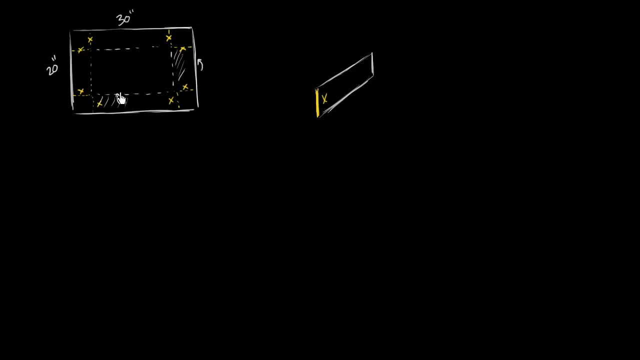 If I were to fold this flap right over here, if I were to fold that up, then it would look like this. It would look like this: My best attempt to draw it. It would look like that And then I would fold that back, flap up. 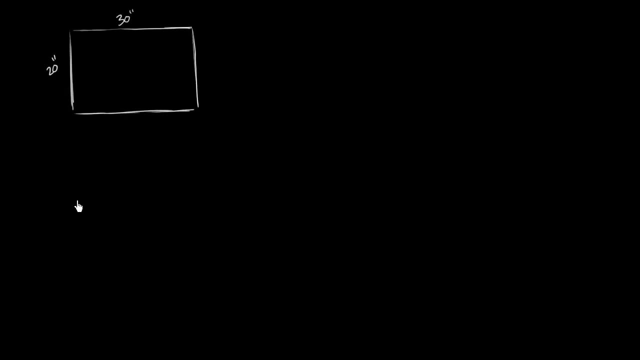 it is 20 inches by 30 inches And what we're going to do is cut out the corners of this cardboard, And all the corners are going to be squares, And we're going to cut out an x by x corner from each of the corners of this piece of cardboard. 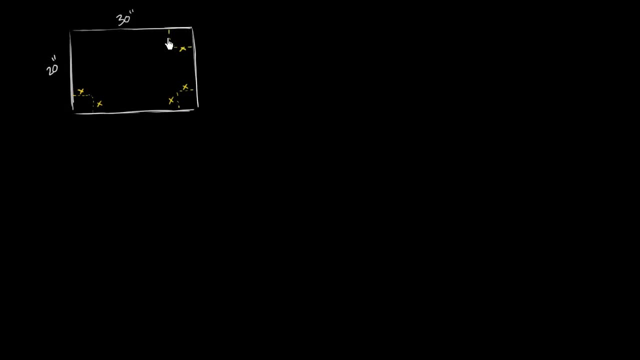 x by x, Over here, x by x, And then over here, x by x. And what we'll do is, after we cut out those corners, we can essentially fold down the flaps. Let me draw the flaps so you can imagine. 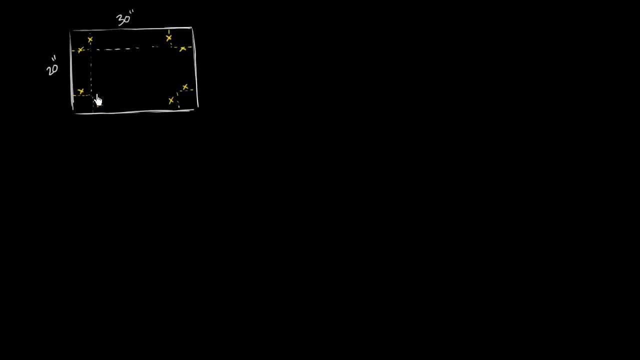 We can fold right there, We could fold right there, We could fold right there And we would form. I guess you could imagine a box without a bottom to it, Or you could view a box without a top to it. So if we were to fold everything up, 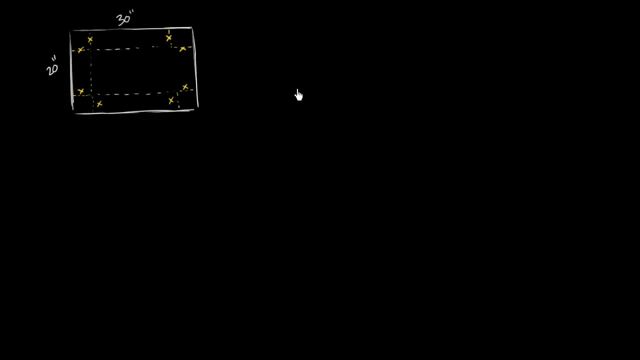 we would get a container that looks something like this. Let me make my best attempt to draw it So it would look like this. It would look like this: This is one flap folded up. You can imagine this flap right over here If I were to fold it up like that. 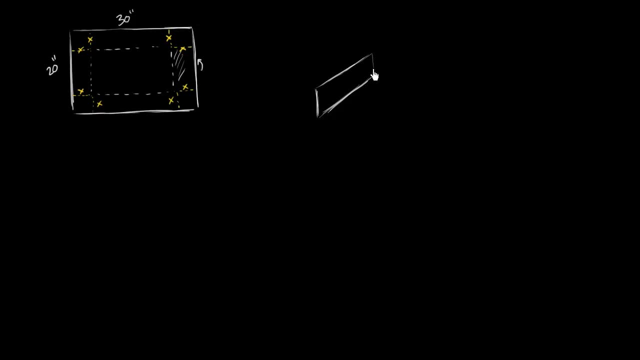 it now would look like this. It would now look like this: The height of the flap is x, So this distance right over here is x. And then if I were to fold this flap, if I were to, let me do that a little bit neater. 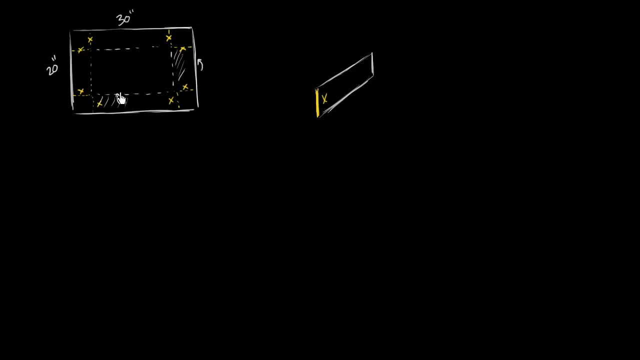 If I were to fold this flap right over here, if I were to fold that up, then it would look like this. It would look like this: My best attempt to draw it. It would look like that And then I would fold that back, flap up. 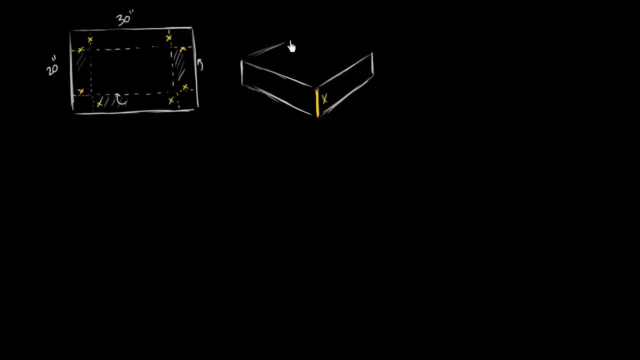 So the back flap would look something like that. That would be the back flap. It would look something like that. And then this flap over here would, if I fold it up, would look something like: would look something like that. And then, of course, my base of my whole thing. 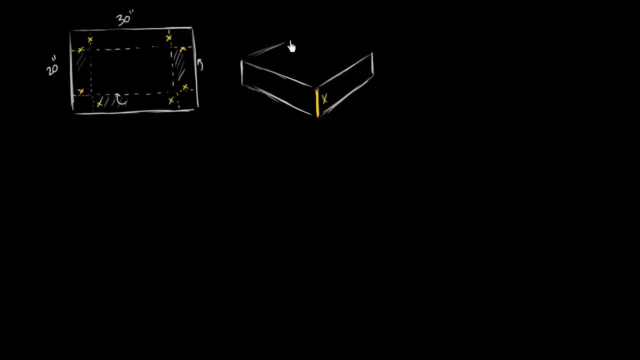 So the back flap would look something like that. That would be the back flap. It would look something like that. And then this flap over here would, if I fold it up, would look something like: would look something like that. And then, of course, my base of my whole thing. 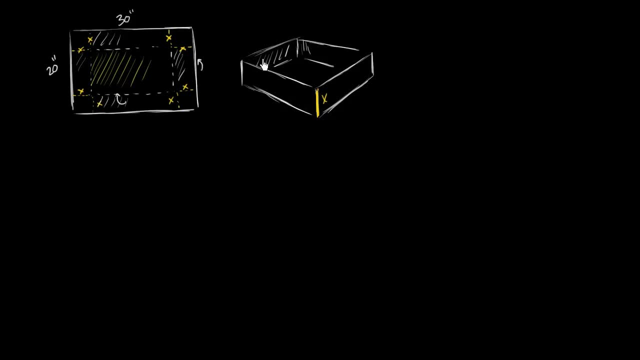 so this whole region right over here of my piece of cardboard would be the back flap, The floor would be the floor of this box that I'm constructing, And what I want to do is I want to maximize the volume of this box, I want to maximize how much it can hold. 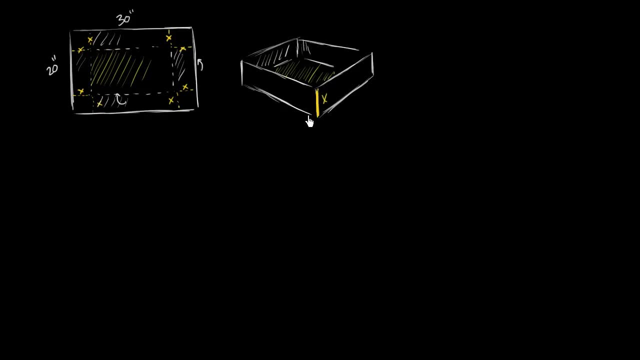 And I want to maximize it by picking my x appropriately. So let's think about what the volume of this box is as a function of x. Well, in order to do that, we have to figure out all the dimensions of this box as a function of x. 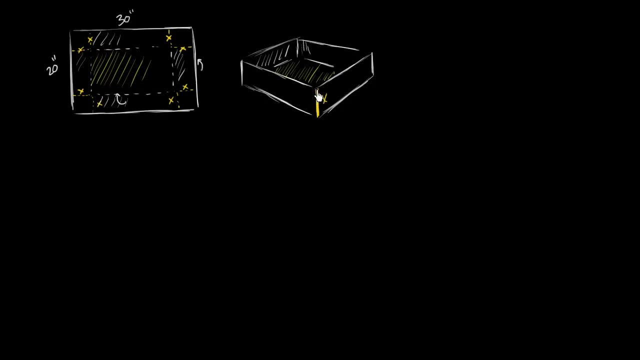 We already know that this corner right over here, which is made up of when this side and this side connect, when you fold these two flaps up, that's going to be the same height over there. That's going to be the same height over there. 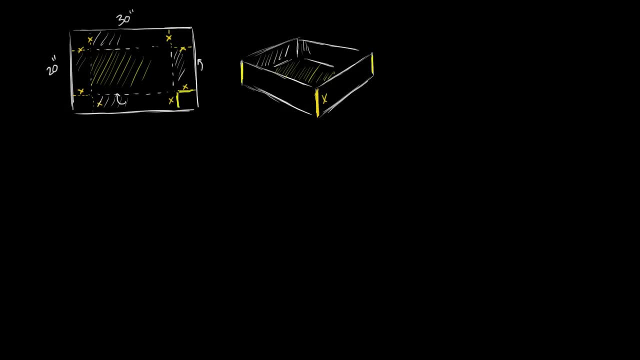 The height of this box is going to be x, But what's the width? What is the width of this box going to be? Well, the width of the box is going to be this distance, right over here, And this distance is going to be 20, 20 inches. 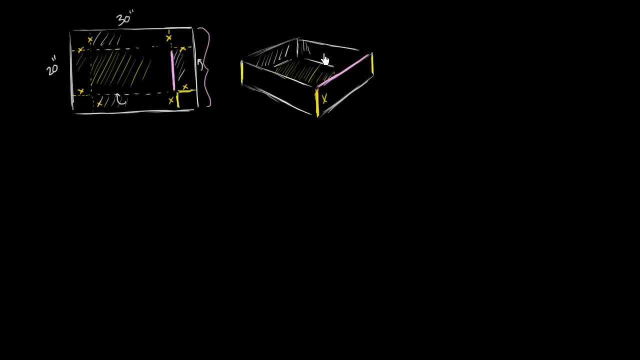 minus not 1x, but minus 2x's. So this is going to be 20, 20 minus 2x. You see it right over here. This whole distance is 20.. You subtract this x. you subtract this x. 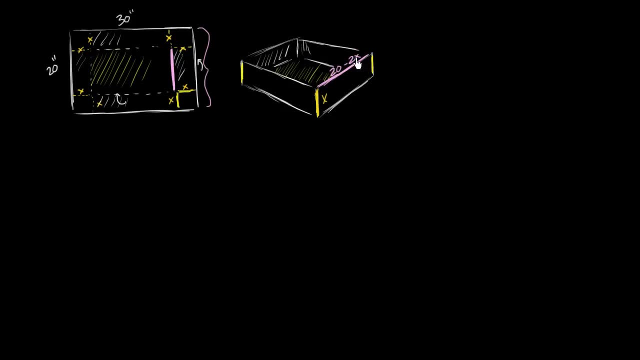 and you get this distance right over here. So it's 20 minus 2x. Now, the same logic. the same logic. what is the depth of the box? What is that distance right over there? Well, that distance is this distance. 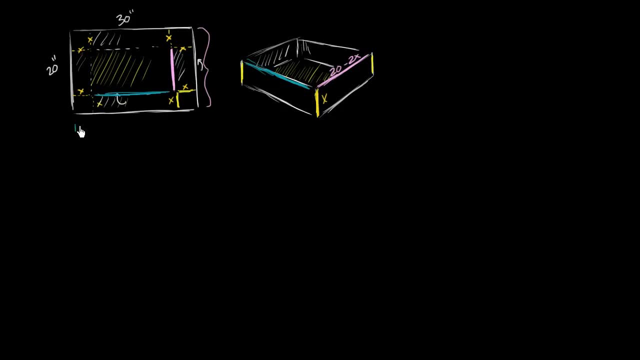 is this distance right over here? We know that this entire distance is 30 inches. If we subtract out this distance, this x, and we subtract out this x, we get the distance that we care about. So this is going to be 30,. 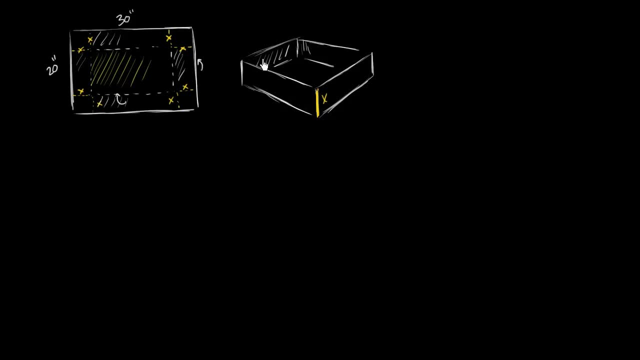 so this whole region right over here of my piece of cardboard would be the back flap, The floor would be the floor of this box that I'm constructing, And what I want to do is I want to maximize the volume of this box, I want to maximize how much it can hold. 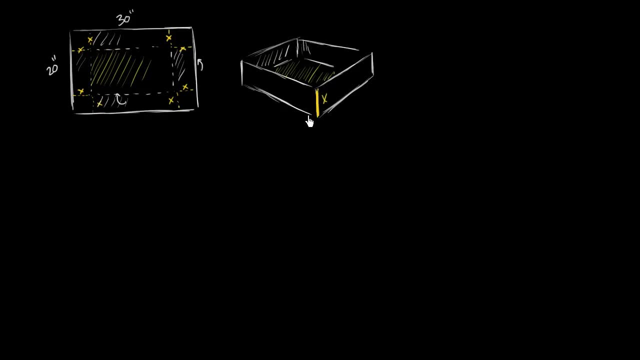 And I want to maximize it by picking my x appropriately. So let's think about what the volume of this box is as a function of x. Well, in order to do that, we have to figure out all the dimensions of this box as a function of x. 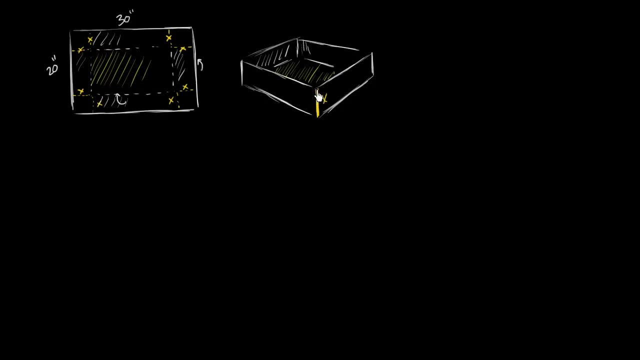 We already know that this corner right over here, which is made up of when this side and this side connect, when you fold these two flaps up, that's going to be the same height over there. That's going to be the same height over there. 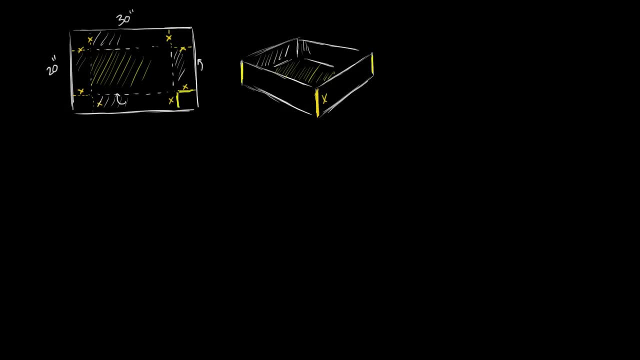 The height of this box is going to be x, But what's the width? What is the width of this box going to be? Well, the width of the box is going to be this distance, right over here, And this distance is going to be 20, 20 inches. 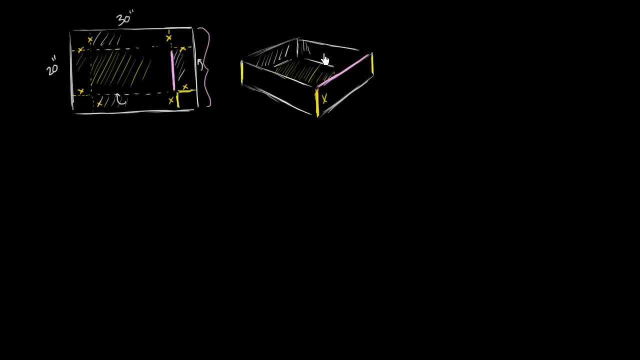 minus not 1x, but minus 2x. So this is going to be 20, 20 minus 2x. You see it right over here. This whole distance is 20.. You subtract this x. you subtract this x. 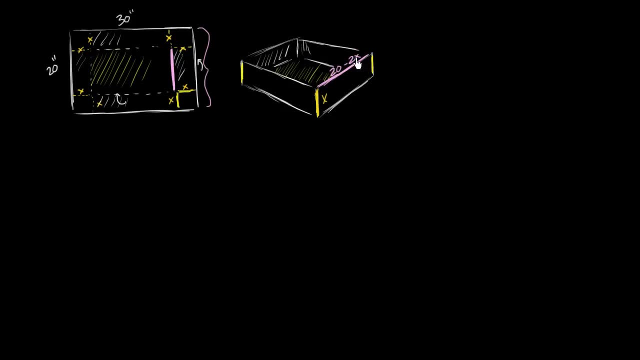 and you get this distance right over here. So it's 20 minus 2x. Now, the same logic. the same logic. what is the depth of the box? What is that distance right over there? Well, that distance is this distance. 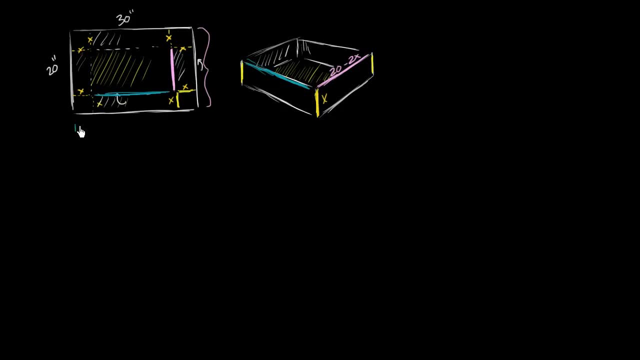 is this distance right over here? We know that this entire distance is 30 inches. If we subtract out this distance, this x, and we subtract out this x, we get the distance that we care about. So this is going to be 30,. 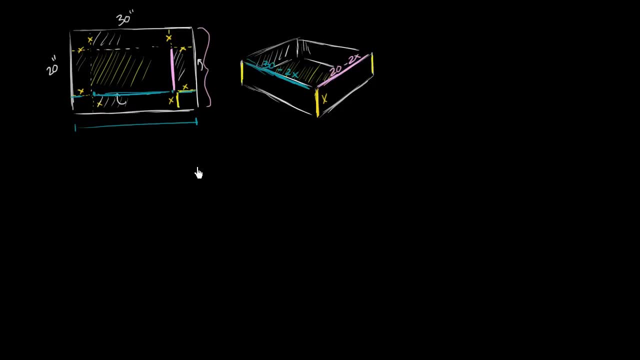 30 minus 2x. So now we have all of the dimensions. So what would the volume be as a function of x? Well, the volume, the volume as a function of x, is going to be equal to the height, which is x. 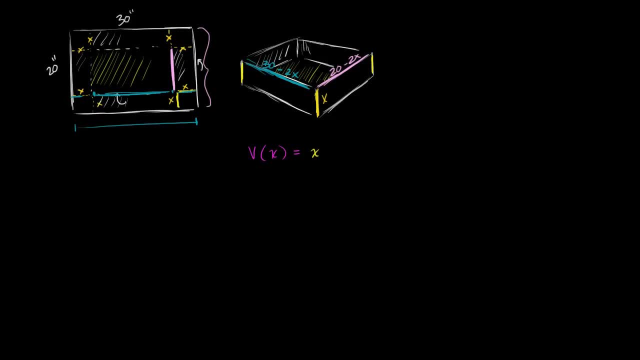 the height, which is x times the width, which is 20 minus x 20, sorry, 20 minus 2x- times the depth, which is 30 minus 2x, which is 30 minus 2x. 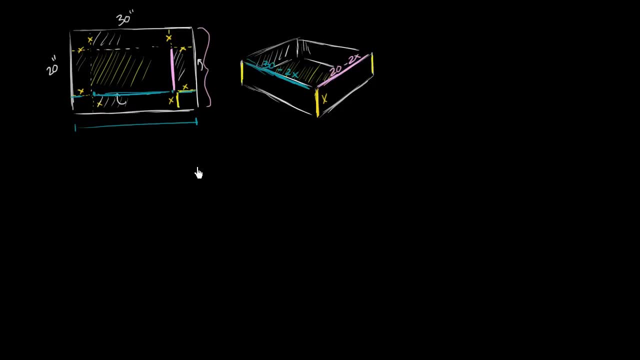 30 minus 2x. So now we have all of the dimensions. So what would the volume be as a function of x? Well, the volume, the volume as a function of x, is going to be equal to the height, which is x. 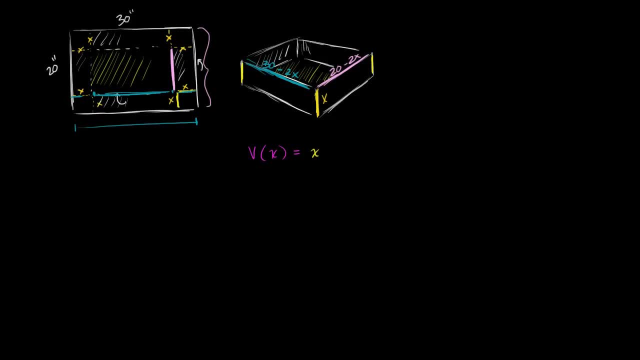 the height, which is x times the width, which is 20 minus x 20, sorry, 20 minus 2x- times the depth, which is 30 minus 2x, which is 30 minus 2x. 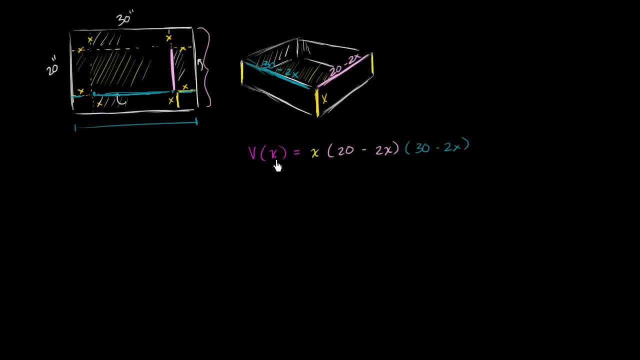 Now, what are possible values of x that give us a valid volume? Well, x can't be, x can't be less than 0.. You can't make a negative cut here. Somehow we would have to add cardboard or something there. So we know that x is going to be greater than or equal to 0. 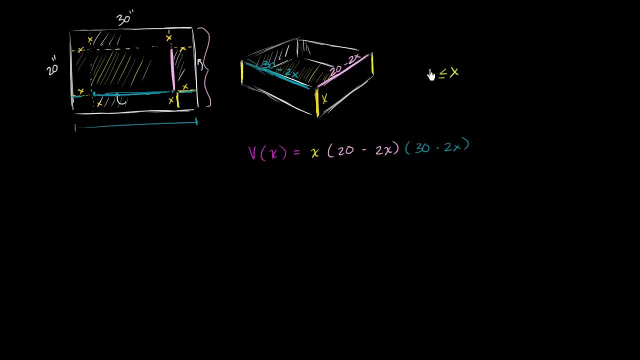 So let me write this down: x is going to be greater than or equal to 0. And what does it have to be less than? Well, I can cut at most. we can see here the length, right over here, this pink color. 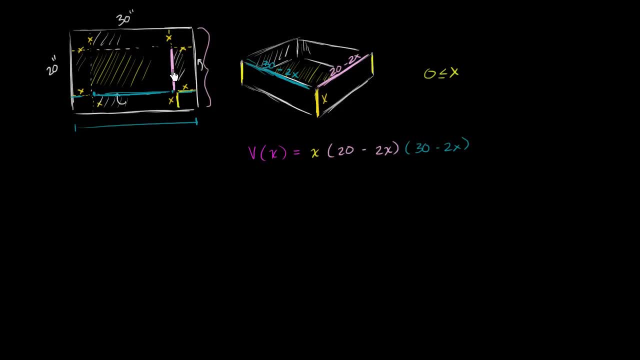 this mauve color is 20 minus 2x, So this has got to be greater than 0.. This is always going to be shorter than the 30 minus 2x, But the 20 minus 2x has to be greater than. 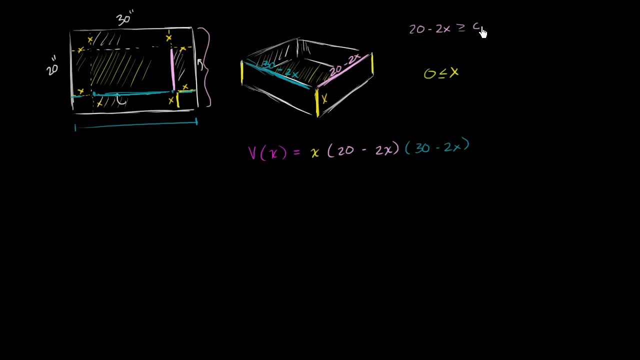 has to be greater than or equal to 0.. You can't cut more cardboard than there is. Or you could say that 20 has to be greater than or equal to 2x, Or you could say that 10 is going to be greater than or equal to x. 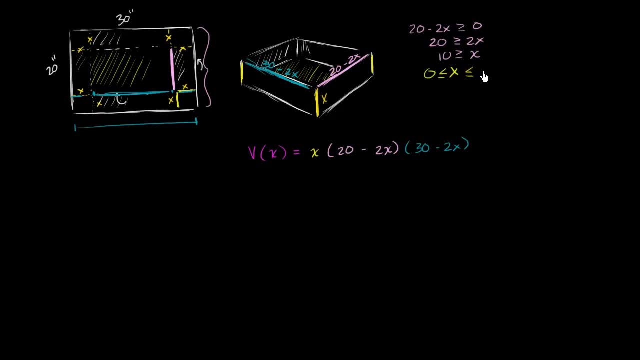 which is another way of saying that x is going to be less than or equal to 10.. It's a different shade of yellow. x is going to be less than or equal to 10.. So x has got to be between 0 and 10.. 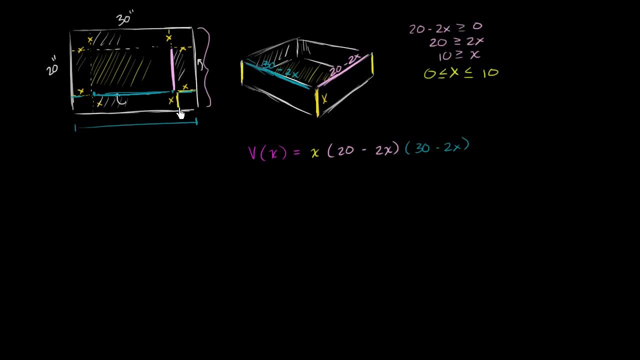 Otherwise we've cut too much or we're somehow adding cardboard or something. So first let's think about the volume, at the end points of this, of our- essentially of our- domain, of what x can be for our volume. Well, our volume. 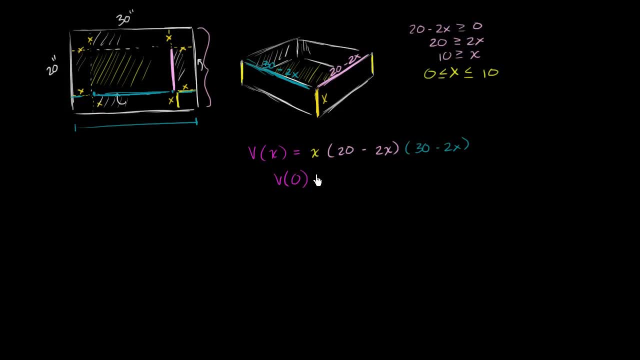 our volume, when x is equal to 0, is equal to what We can have, 0 times all of this stuff. and it's pretty obvious: You're not going to have any height here, So you're not going to have any volume, So our volume would be 0.. 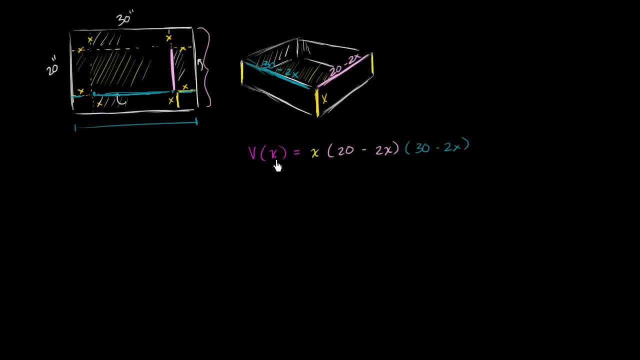 Now, what are possible values of x that give us a valid volume? Well, x can't be, x can't be less than 0.. You can't make a negative cut here. Somehow we would have to add cardboard or something there. So we know that x is going to be greater than or equal to 0. 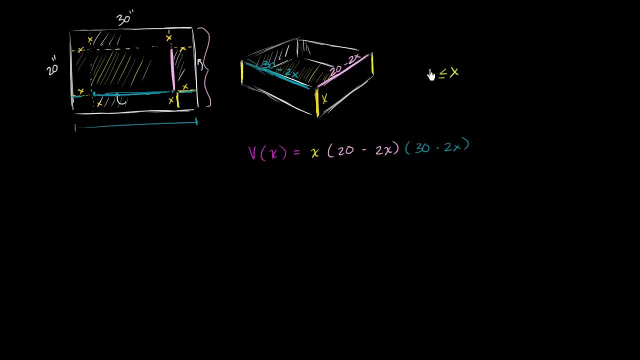 So let me write this down: x is going to be greater than or equal to 0. And what does it have to be less than? Well, I can cut at most. we can see here the length, right over here, this pink color. 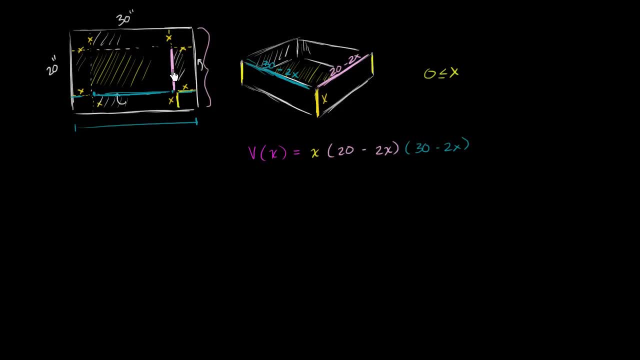 this mauve color is 20 minus 2x, So this has got to be greater than 0.. This is always going to be shorter than the 30 minus 2x, But the 20 minus 2x has to be greater than. 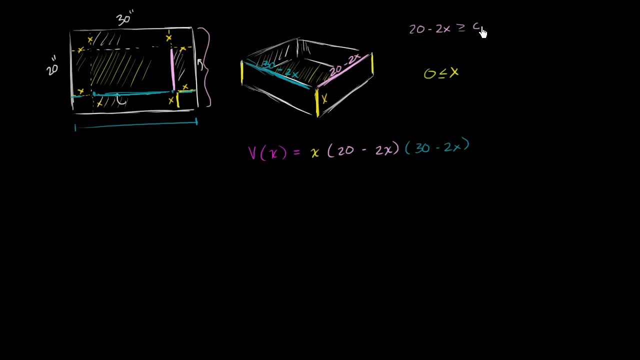 has to be greater than or equal to 0.. You can't cut more cardboard than there is. Or you could say that 20 has to be greater than or equal to 2x, Or you could say that 10 is going to be greater than or equal to x. 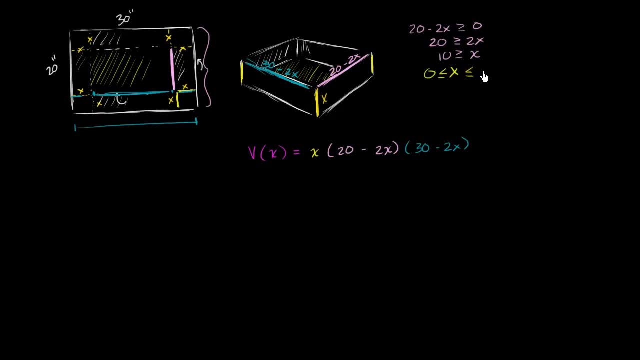 which is another way of saying that x is going to be less than or equal to 10.. It's a different shade of yellow. x is going to be less than or equal to 10.. So x has got to be between 0 and 10.. 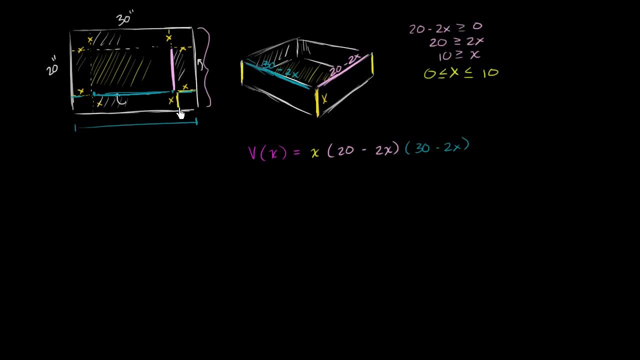 Otherwise we've cut too much or we're somehow adding cardboard or something. So first let's think about the volume, at the end points of this, of our- essentially of our- domain, of what x can be for our volume. Well, our volume. 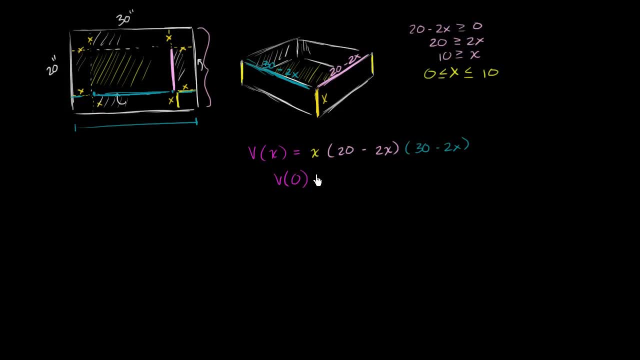 our volume, when x is equal to 0, is equal to what We can have, 0 times all of this stuff. and it's pretty obvious: You're not going to have any height here, So you're not going to have any volume, So our volume would be 0.. 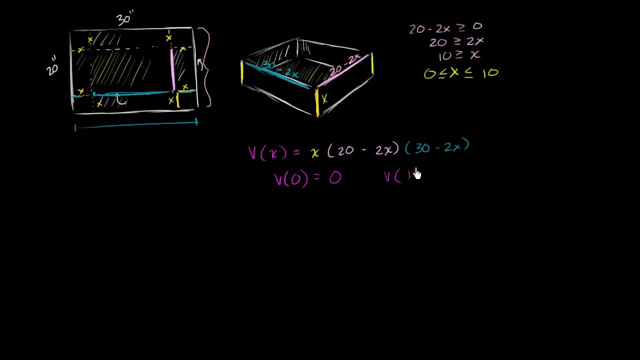 What is our volume when x is equal to 10?? Well, if x equaled 10, then the width here that I've drawn in pink would be 0.. So, once again, we would have no volume And this term right over here. 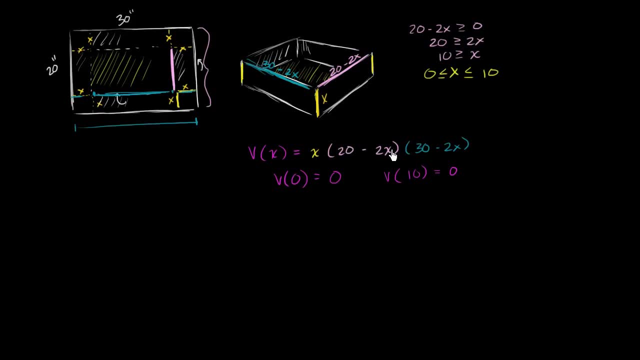 if we just look at it, if we look at it algebraically, would also be equal to 0. So this whole thing would be equal to 0. So some place in between x equals 0 and x equals 10, we should achieve our maximum volume. 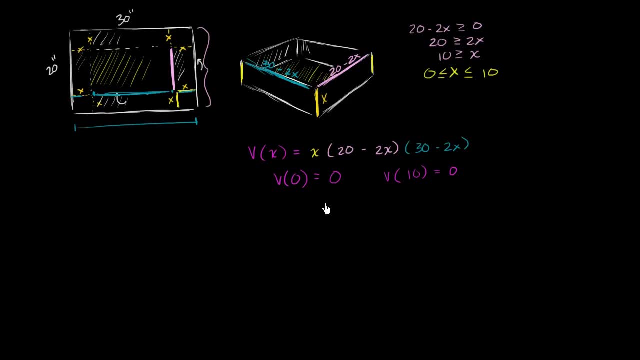 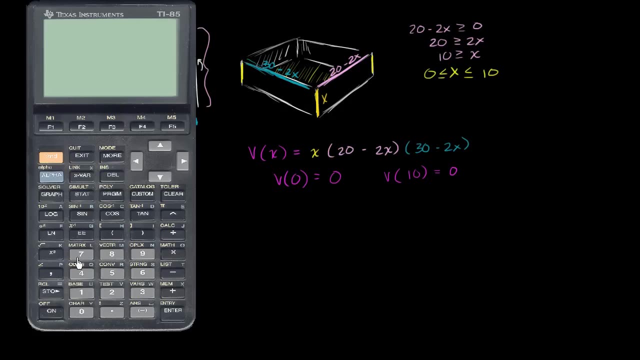 And before we do it analytically with a bit of calculus, let's do it graphically. So I'll get my handy TI-85 out. So let me get my TI-85 out. And so first let me set my range appropriately. 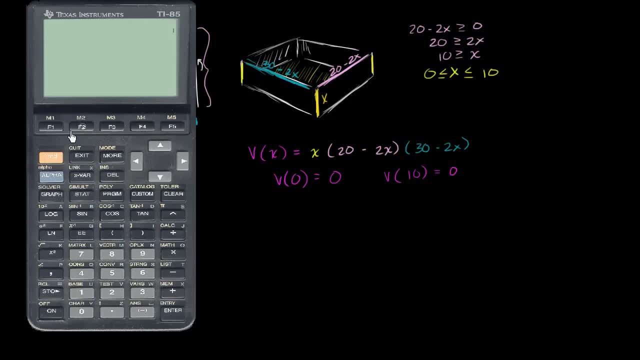 before I attempt to graph it. So I'll put my graph function. Let me set my range. So my minimum x value, let me make that 0.. We know that x cannot be less than 0.. My maximum x value: well, 10 seems pretty good. 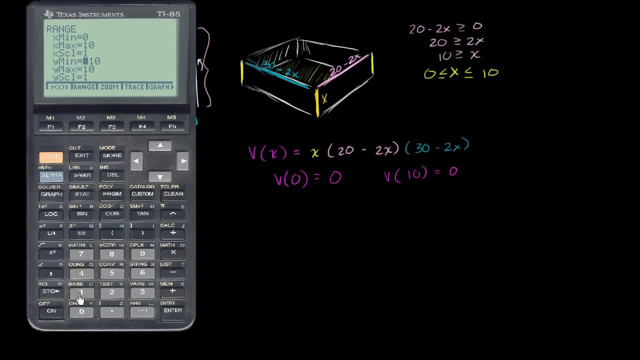 My minimum y value. this is essentially going to be my volume. I'm not going to have negative volume, so let me set that equal 0. And my maximum y value. let's see what would be reasonable here. I'm just going to pick a random x. 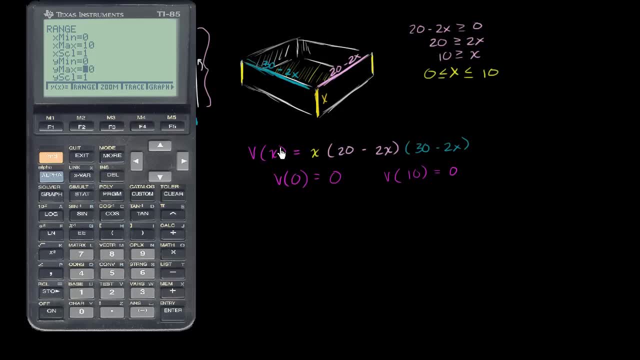 and see what type of a volume I get. So if x were to be 5, it would be 5 times 20 minus 10, which is 10.. So that would be: did I do that right? Yeah, 20 minus 2 times 5,. 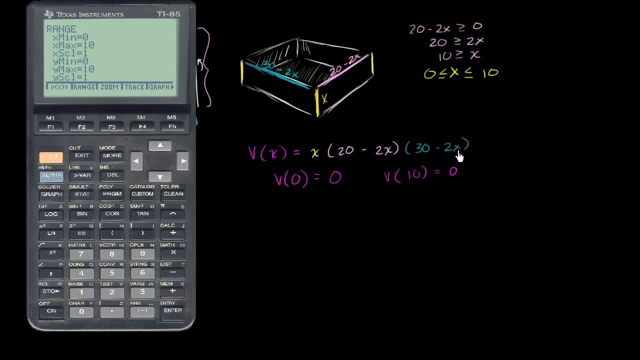 so that would be 10.. And then times 30 minus 2 times 5, which would be 20.. So it would be 5 times 10 times 20.. So you'd get a volume of 1,000 cubic inches. 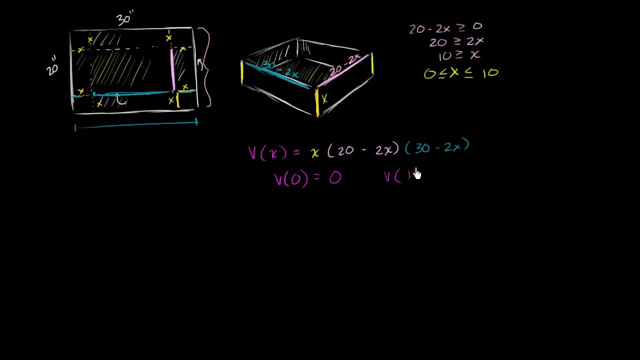 What is our volume when x is equal to 10?? Well, if x equaled 10, then the width here that I've drawn in pink would be 0.. So, once again, we would have no volume And this term right over here. 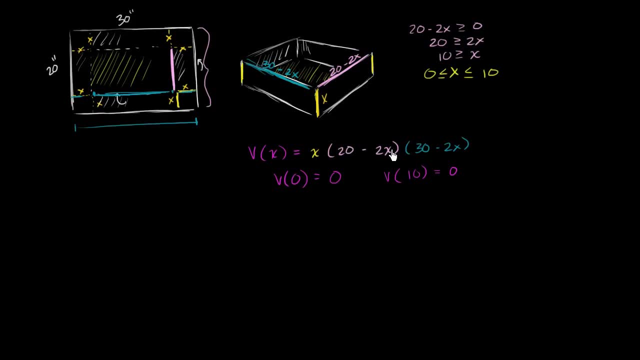 if we just look at it, if we look at it algebraically, would also be equal to 0. So this whole thing would be equal to 0. So some place in between x equals 0 and x equals 10, we should achieve our maximum volume. 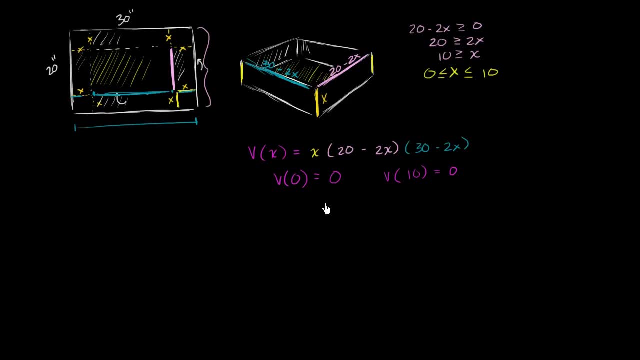 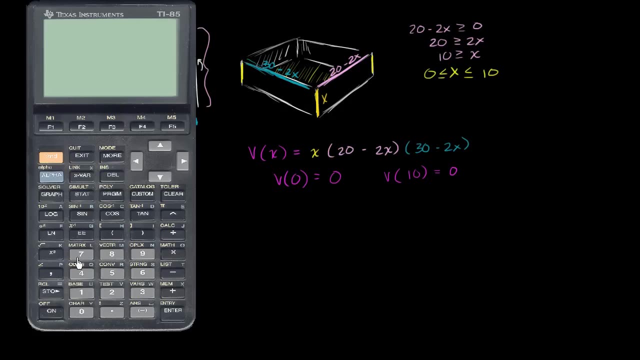 And before we do it analytically with a bit of calculus, let's do it graphically. So I'll get my handy TI-85 out. So let me get my TI-85 out. And so first let me set my range appropriately. 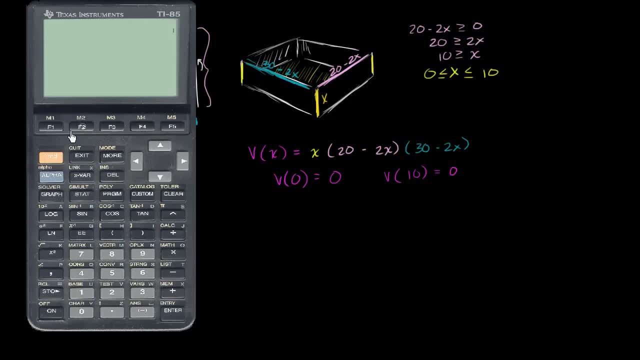 before I attempt to graph it. So I'll put my graph function. Let me set my range. So my minimum x value, let me make that 0.. We know that x cannot be less than 0.. My maximum x value: well, 10 seems pretty good. 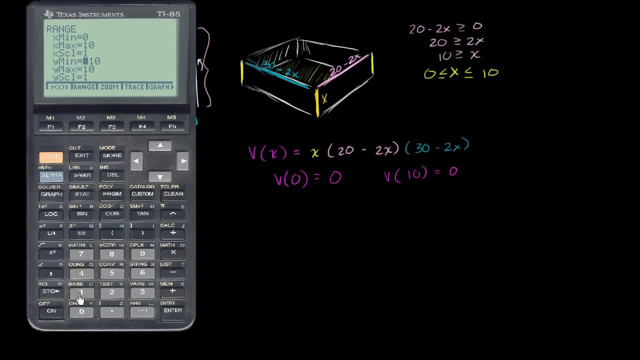 My minimum y value. this is essentially going to be my volume. I'm not going to have negative volume, so let me set that equal 0. And my maximum y value. let's see what would be reasonable here. I'm just going to pick a random x. 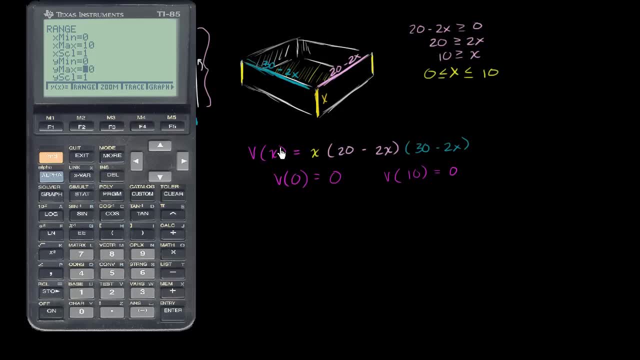 and see what type of a volume I get. So if x were to be 5, it would be 5 times 20 minus 10, which is 10.. So that would be: did I do that right? Yeah, 20 minus 2 times 5,. 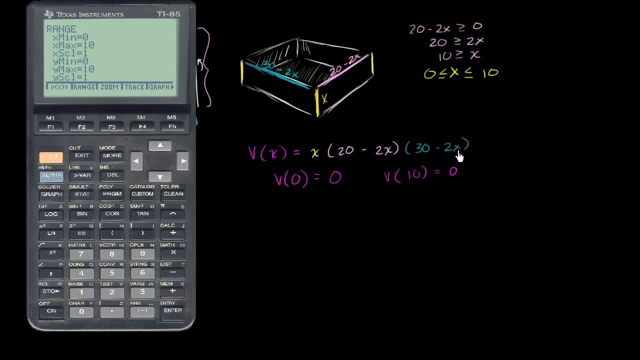 so that would be 10.. And then times 30 minus 2 times 5, which would be 20.. So it would be 5 times 10 times 20.. So you'd get a volume of 1,000 cubic inches. 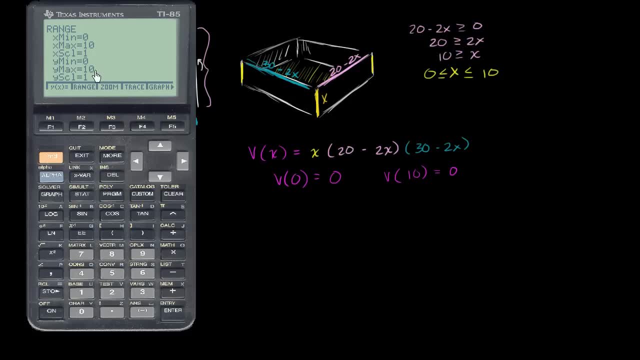 And I just randomly picked the number 5.. So let me give my maximum y value a little higher than that, just in case that that isn't the maximum value I just randomly picked. So let's say y max is 1,500. 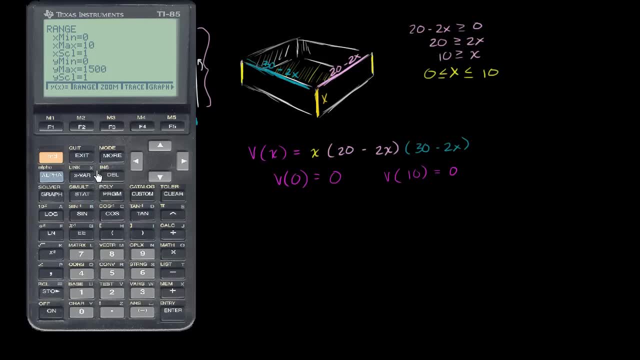 And if, for whatever reason, our graph doesn't fit in there, then maybe we can make our y max even larger. So I think this is going to be a decent range. Now let's actually input the function itself. So our volume is equal to. 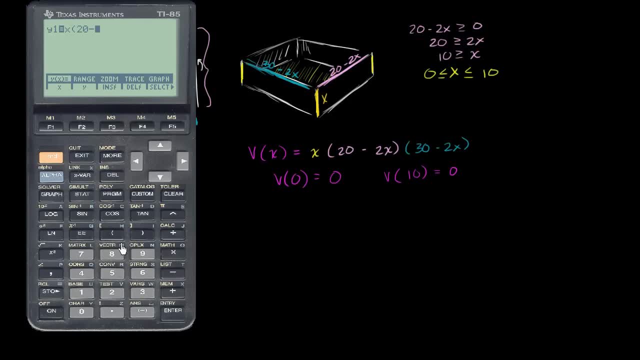 x times 20 minus 2x, times 30 minus 2x, And that looks about right. So now I think we can graph it. So second- and I want to select that up there, so I'll do graph- And it looks like we did get the right range. 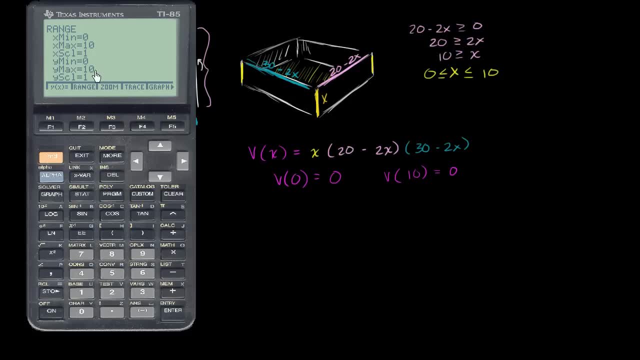 And I just randomly picked the number 5.. So let me give my maximum y value a little higher than that, just in case that that isn't the maximum value I just randomly picked. So let's say y max is 1,500. 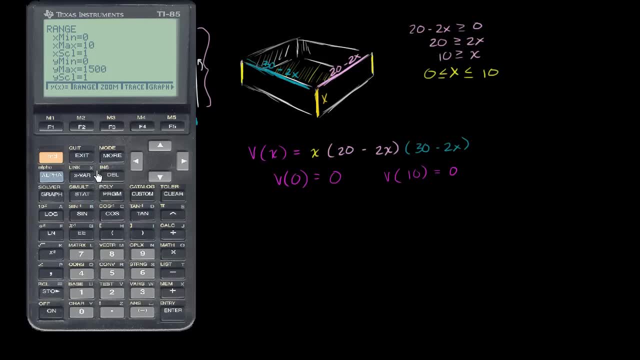 And if, for whatever reason, our graph doesn't fit in there, then maybe we can make our y max even larger. So I think this is going to be a decent range. Now let's actually input the function itself. So our volume is equal to. 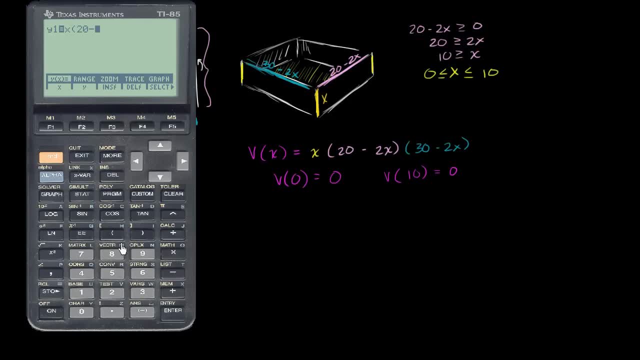 x times 20 minus 2x, times 30 minus 2x, And that looks about right. So now I think we can graph it. So second- and I want to select that up there, so I'll do graph- And it looks like we did get the right range. 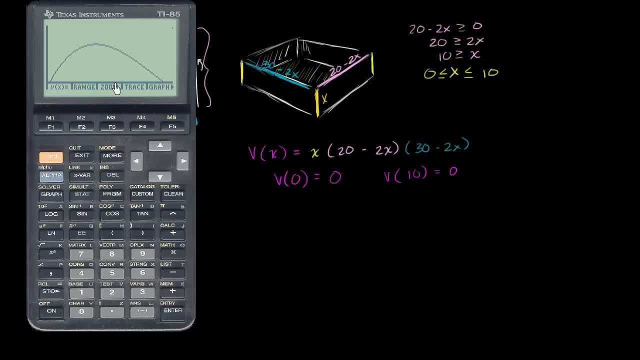 So this tells us volume is a function of x, between x is 0 and x is 10.. And it does look like we hit a maximum point right around there. So what I'm going to do is I'm going to use the trace function. 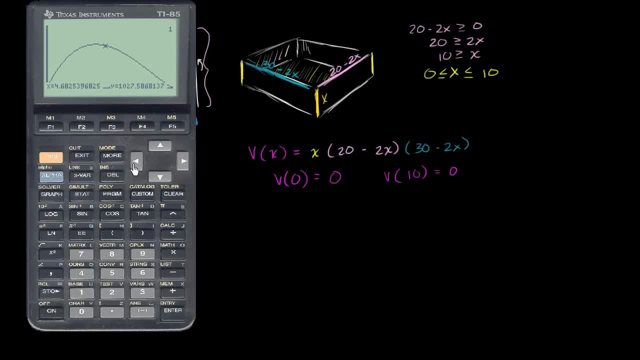 to figure out roughly what that maximum point is. So let me trace this function so I can still go higher, higher. OK, So over there my volume is 1055.5.. Then I can get to 1056.. Then I get to 1056 points.